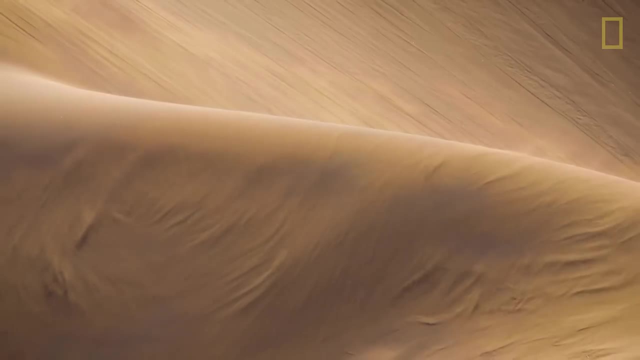 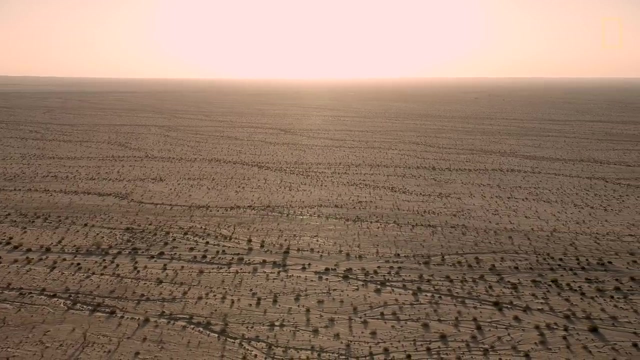 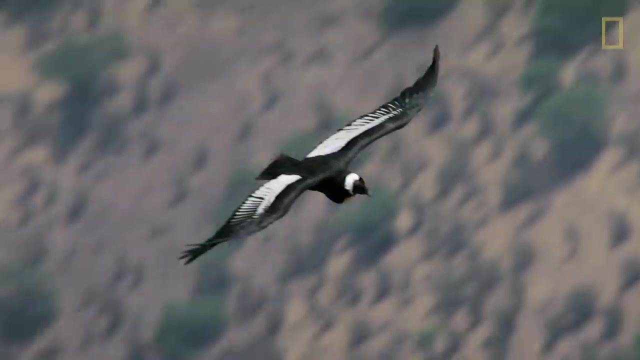 Wind whips over a barren wasteland- vast nothingness as far as the eye can see, or so it may seem. Creatures peek out of burrows, scurry across the sand and soar through the sky, revealing a landscape not as lifeless as it may first appear. 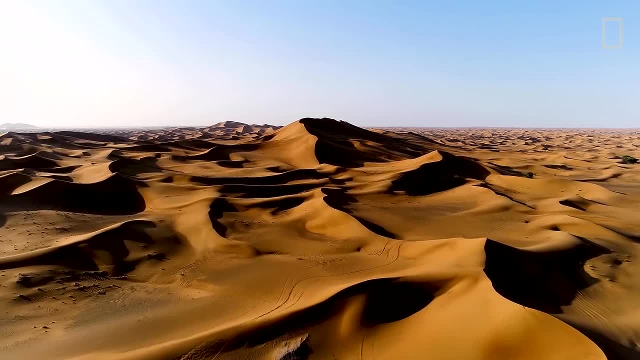 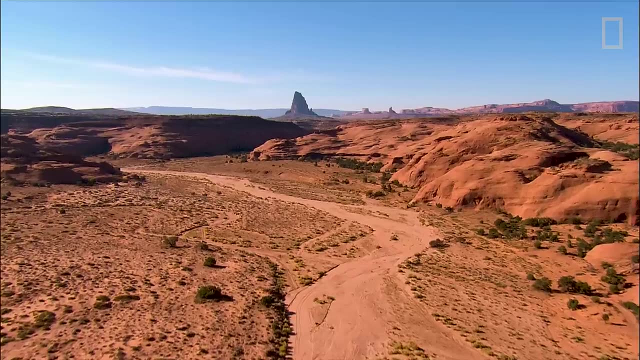 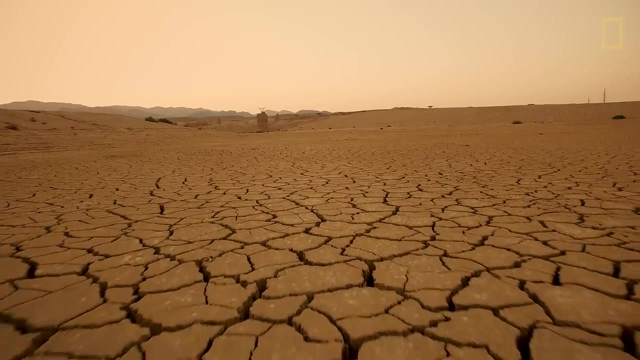 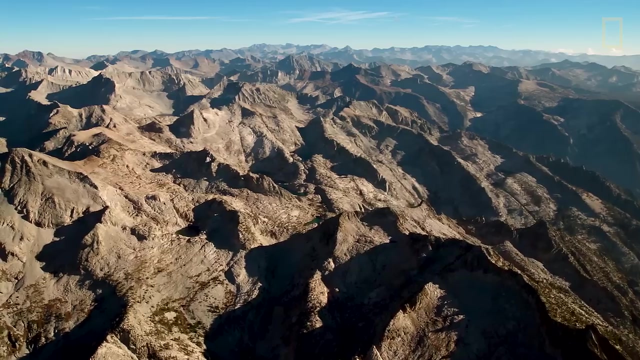 Deserts are often defined as areas of land that receive less than 10 inches of rainfall each year. These regions are low in humidity and can even be moisture deficient, evaporating water faster than it is received. While most deserts are found in the mid-latitudes, these diverse ecosystems occur on all seven continents. 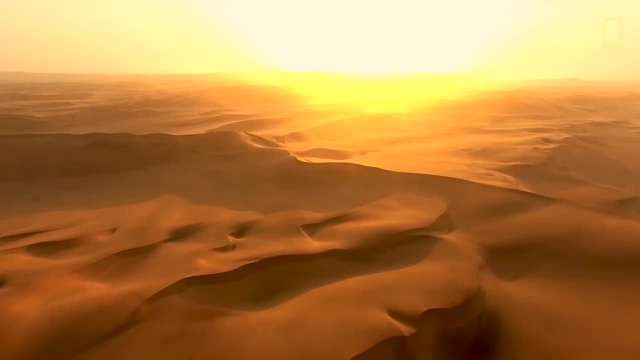 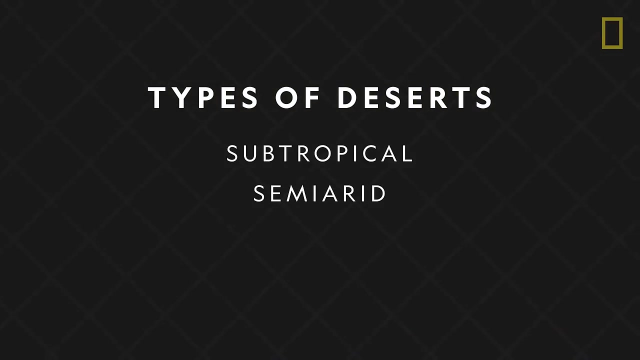 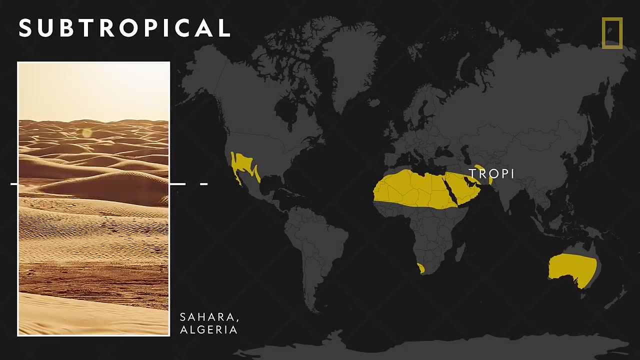 and make up nearly one-third of Earth's total landmass. Deserts are sometimes classified into four major types: subtropical, semi-arid, coastal and polar. Subtropical deserts are found along the equator, in the Tropic of Cancer and the Tropic of Capricorn. 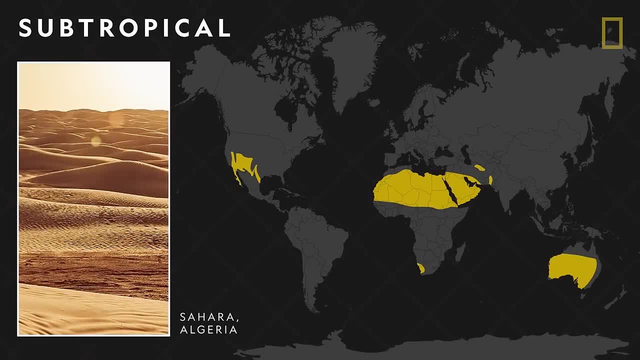 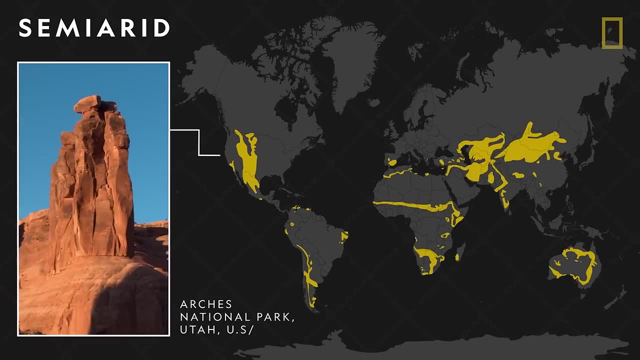 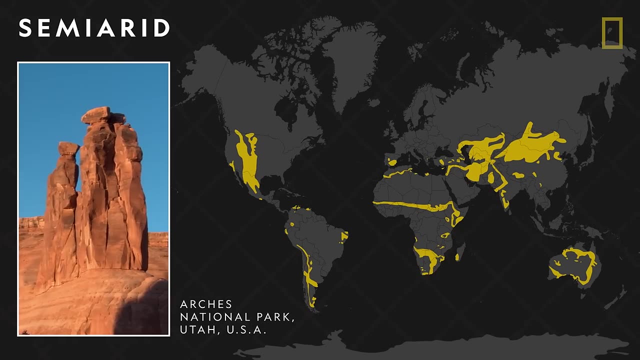 They are the hottest deserts on Earth, with daytime temperatures that can reach up to 120 degrees Fahrenheit. Semi-arid deserts are located in Asia, Europe and North America. These cold winter deserts often fall. These deserts form when tall mountain ranges block moisture through a process called the rain shadow effect. 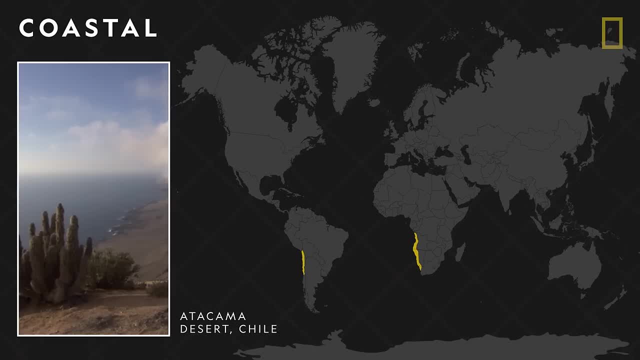 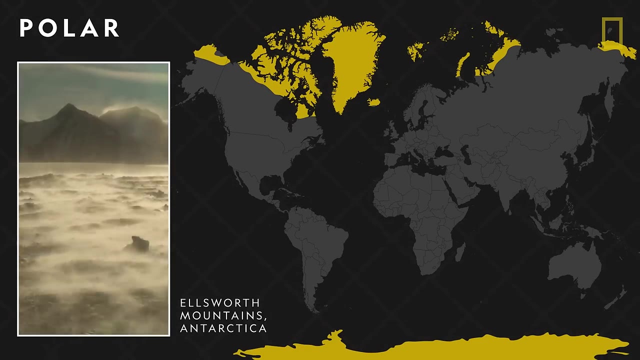 Coastal deserts form alongside the tropical western edges of certain continents. Despite their proximity to water, coastal deserts remain dry. Polar deserts are found in the Arctic and Antarctic, The other end of the extreme winter temperatures in the Antarctic desert average around minus 50 degrees Fahrenheit. 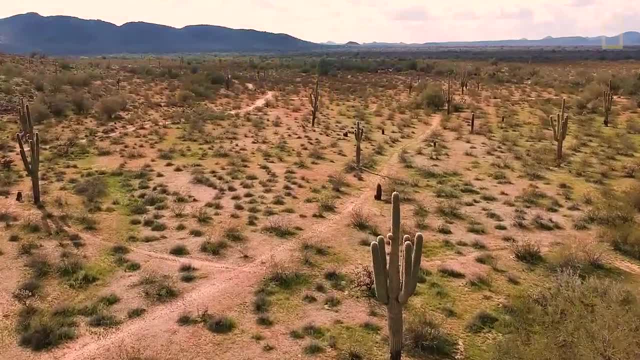 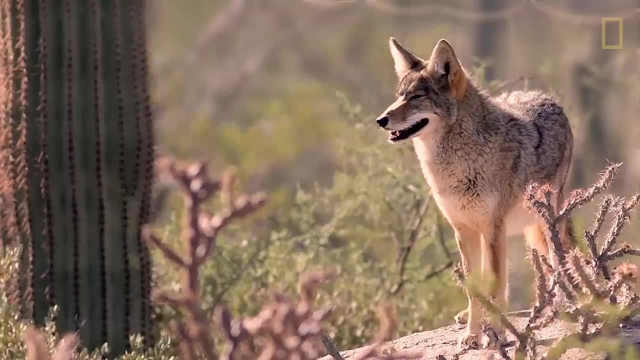 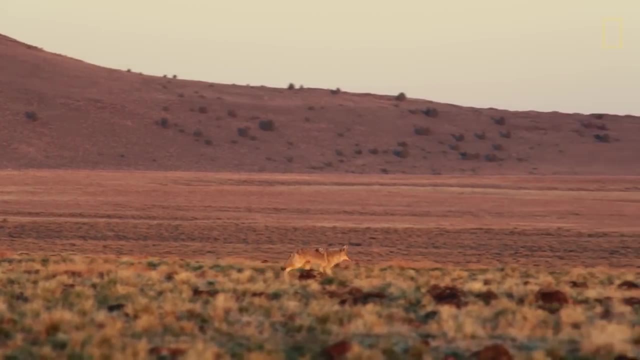 While deserts experience extreme temperatures and receive very little precipitation, they are still important habitats for plants and animals. Desert animals, such as the coyote, have evolved to withstand harsh desert conditions by burrowing into the cool ground and emerging at night when desert temperatures drop. 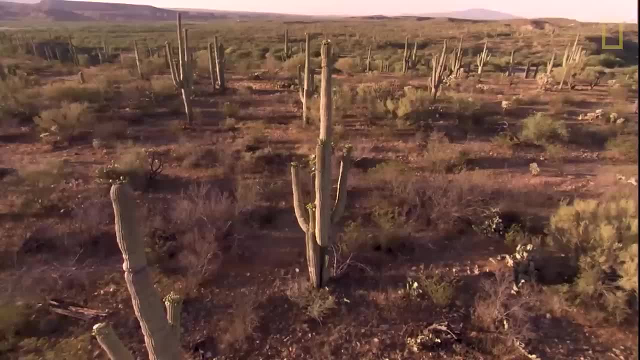 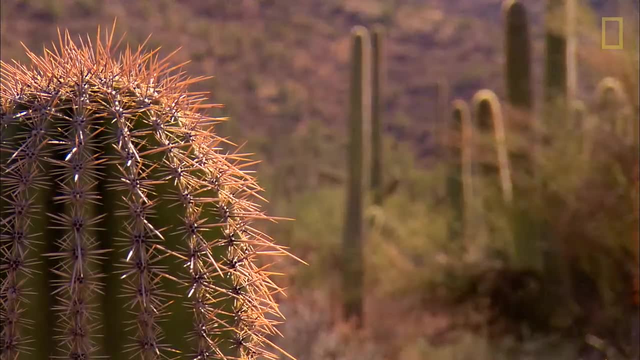 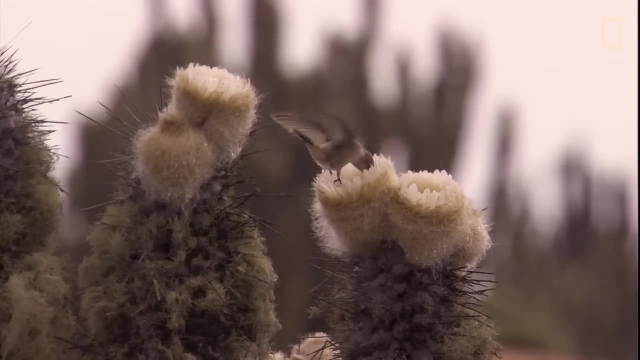 Many desert plants, including the saguaro cactus, have established long and shallow root systems to better absorb what minimal moisture might be Highly specialized to survive in such a harsh environment. desert wildlife is particularly vulnerable to ecological changes. Existing deserts have become less habitable because of rising temperatures.